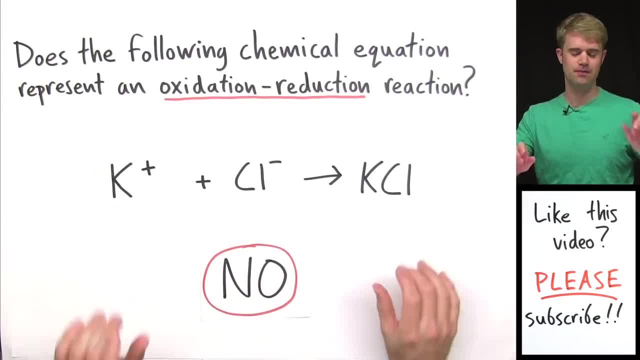 no, This is not an oxidation reduction reaction. So if you got this wrong, I'm not a professional mind reader, but I want to try to read your mind right now and guess why you thought this was a redox reaction. I'm guessing it's because you saw the plus and the minus. 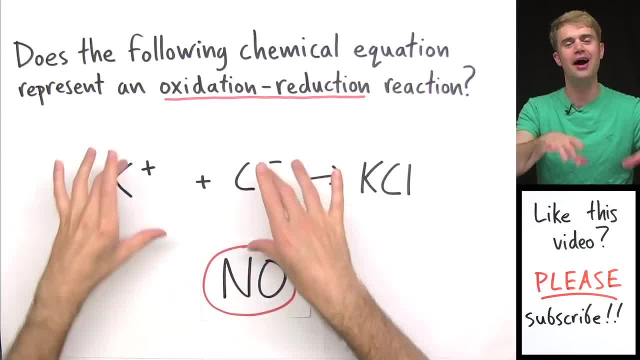 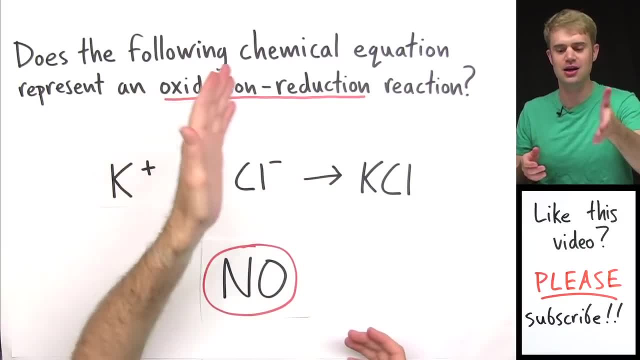 you saw these charges here and you realized we were dealing with a reduction reaction. So you were dealing with ions and you thought, yeah, pluses, minuses, charges, ions- these are things that we see in oxidation reduction reactions. Well, you're half right, We do see. 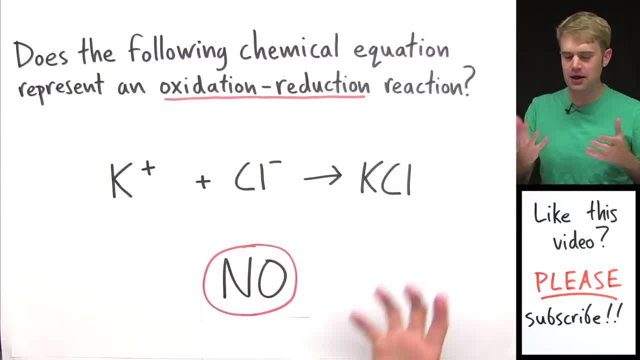 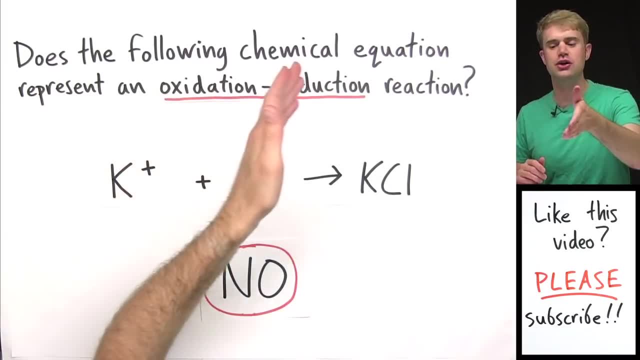 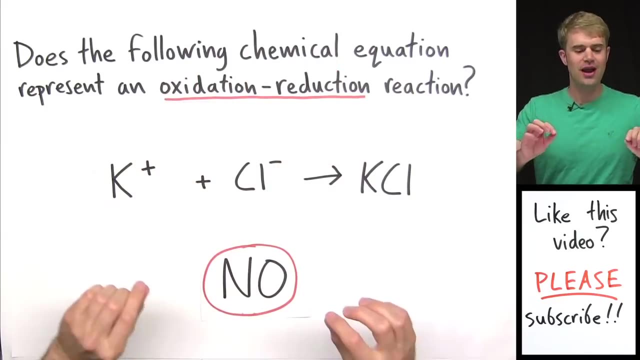 those in oxidation reduction reactions. but just because an equation or a reaction has charges and ions doesn't mean that it has to be an oxidation reduction reaction. Remember what these two words mean. In order for something to be an oxidation reduction reaction, we have to. 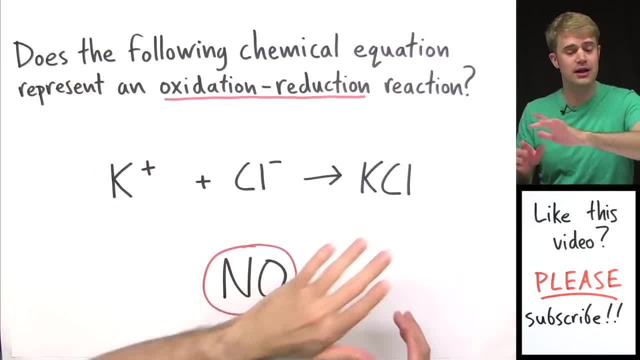 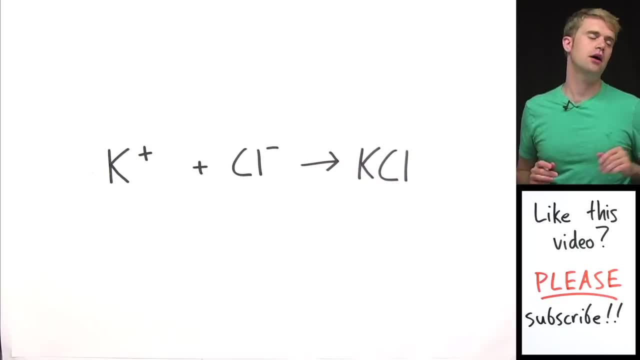 see electrons transferred between atoms. That's not going on here, and let me show you how I know that. So KCl here is an ionic compound, which means that it's made of ions, The K plus ion and the Cl one minus ion. So these atoms have charges and we can even write numbers above these atoms. 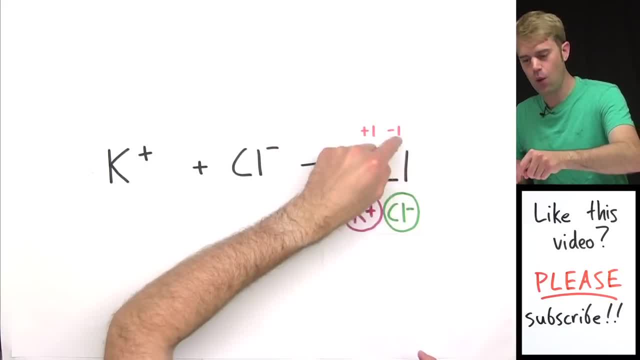 to reinforce. what charge they have? One plus for the K, one minus for the Cl. Now over on this side. let's look at the ionic compound Now. let's look at the ionic compound Now over on this side. 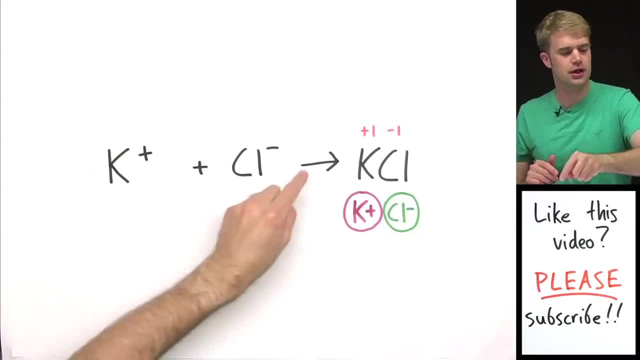 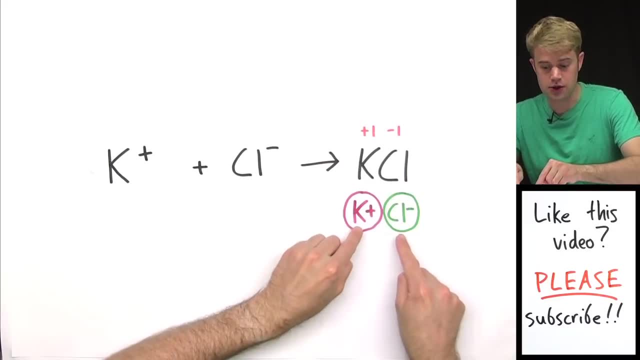 let's look at the ionic compound. Now, over on this side, let's look at the ionic compound. Let's take a look at what's going on. For this to be an oxidation reduction reaction, the K and Cl would have to have a transfer of electrons that create these charges. the plus and the minus. 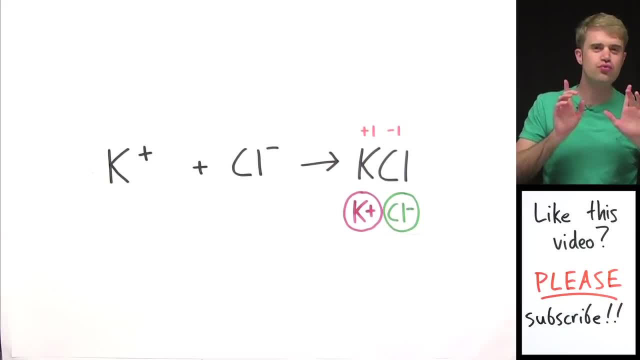 But the atoms over here they already have charges right. K plus: here's a picture of the atom. Cl one minus- here's a picture of the atom And I can put these numbers above them. Got one plus for K one. 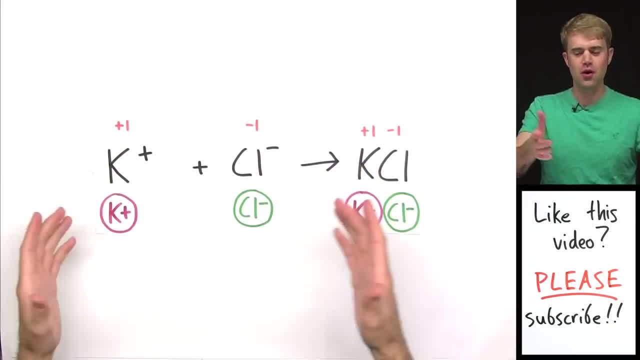 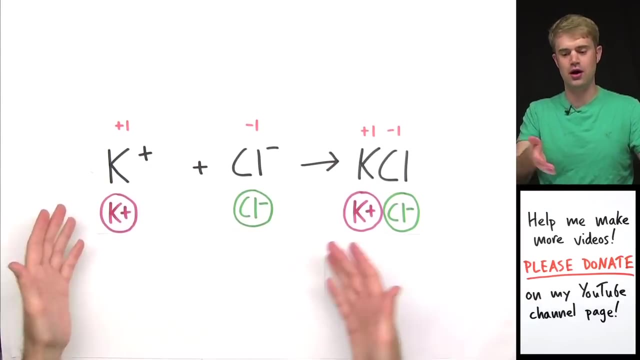 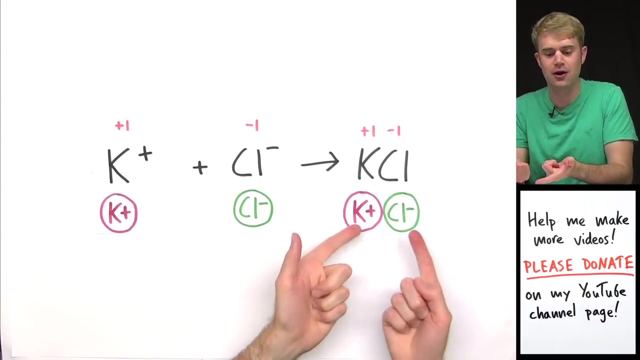 minus or minus one for Cl. So the point of this equation here is that the charges don't change. K and Cl start out plus and minus and they end plus and minus. There's no transfer of electrons that takes place. The only thing that happens is two atoms that started out charged end up sticking together. That's the only thing that's going on in this equation. 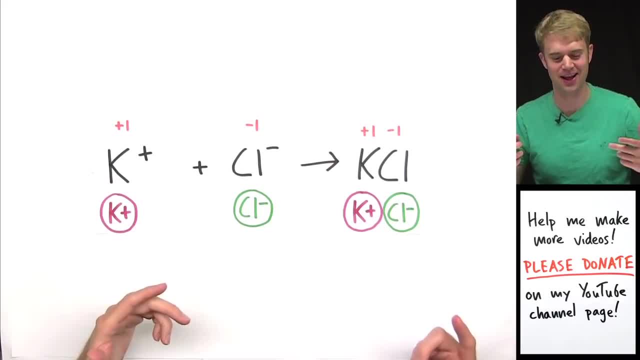 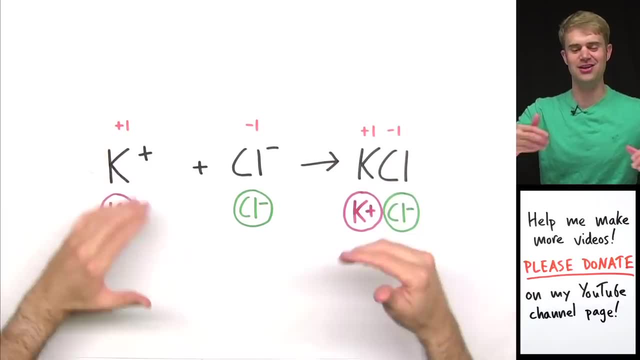 Now, If this still is a little bit confusing, let me show you how we could change this equation to make it actually an oxidation-reduction reaction, And then, when you see the differences, I think this will all make sense. So here's the equation that we said was not a redox reaction. 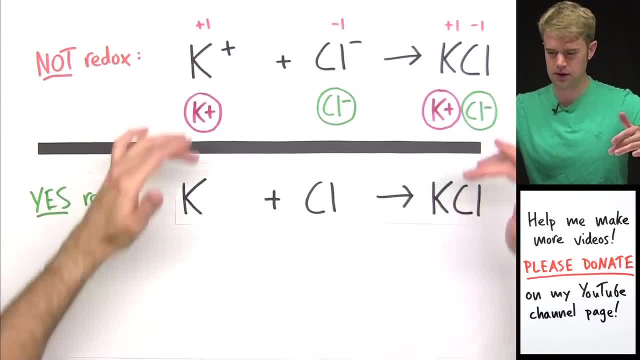 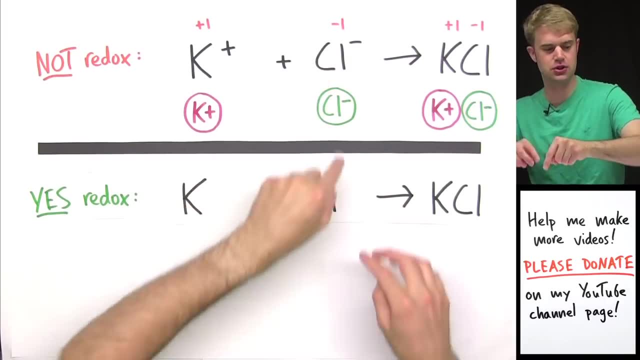 Here's an equation that is a redox reaction. These two reactions look pretty similar, except for one important difference. Take a look at how K and Cl start out. In this equation: up here they had charges. In this equation down here, they don't have charges. 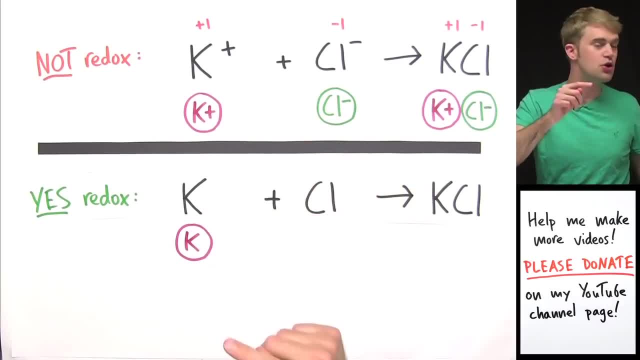 They start out not as K plus and Cl minus, but as neutral atoms, as K and Cl. To emphasize that they're neutral, we can put these oxidation numbers, these zeros, above them. The zeros tell us that they're neutral And then, just like before, KCl is an ionic compound with K plus and Cl minus. 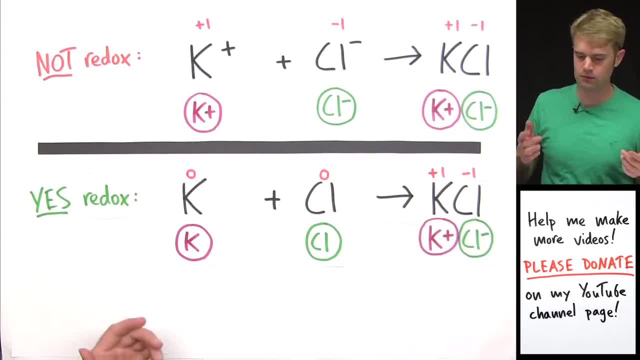 Here are the charges for those atoms. So in order for K and Cl to become K plus and Cl minus, there has to be a transfer of electrons. So what happens is K potassium gives up one of its electrons. It gives it to Cl. 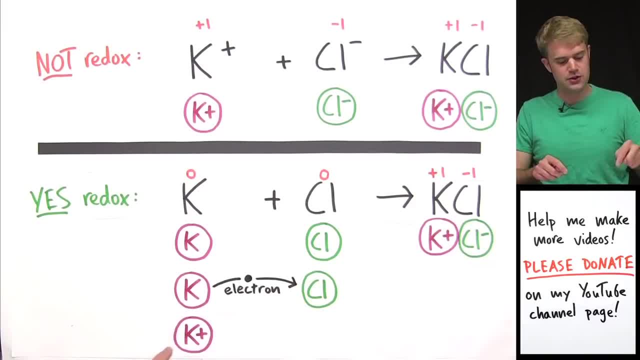 K loses one of its electrons to become K plus or potassium one plus. Cl gains one of these electrons and becomes Cl minus, chloride Cl minus. So now these two atoms end up with charges, but only because of a transfer of electrons. 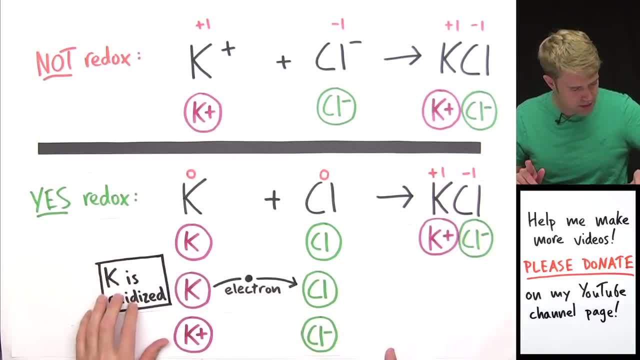 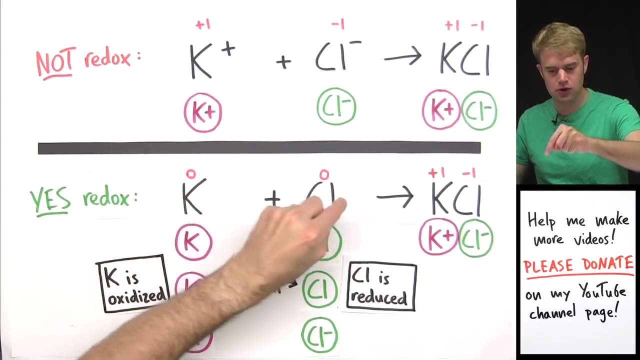 That transfer of electrons caused potassium K to become oxidized And it caused Cl- chlorine- to become reduced. So that's why this is an oxidation reduction reaction, Because potassium and chlorine K and Cl start out neutral. There's a transfer of electrons which gives them charges and then those charges stick together.